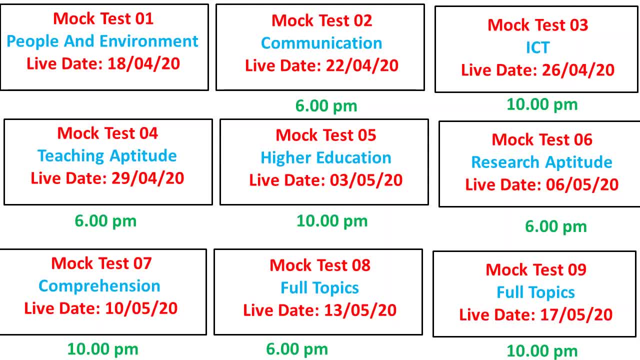 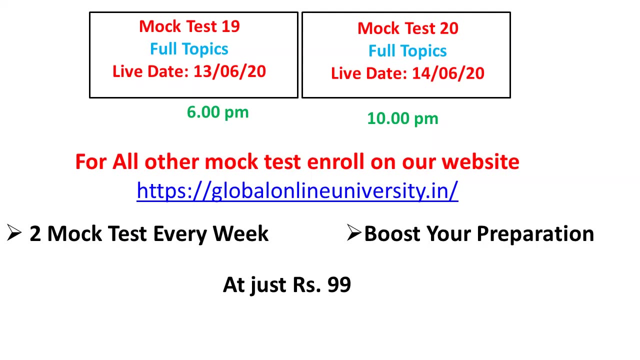 Friends, we have already released the mocktail series on people and environment, on communication, ICT, on teaching aptitude and also on higher education. Our next mocktail series is releasing on research aptitude on 6-5-2020.. Friends, as you all know, we will provide you 20 mocktail series, and these mocktail series will surely boost your preparation. 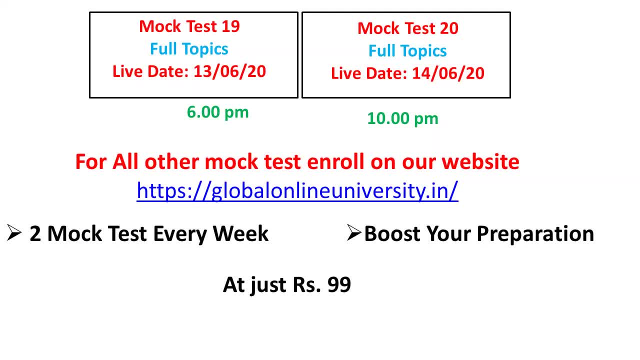 And all these 20 mocktail series will surely boost your preparation. All these mocktail series are available only at Rs 99.. So to get all these mocktail series, go to our website and enroll for the mocktail series. So let us start. 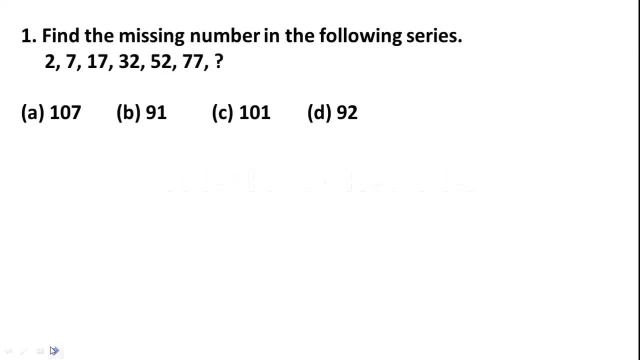 The question is find the missing number in the following series. The series is 2,, 7,, 17,, 32,, 52,, 77.. We have to find the next upcoming series, So options are option A107.. 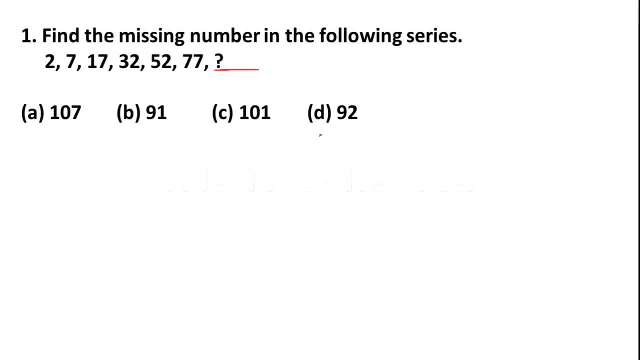 Option B91.. Option C101.. Option D92.. Friends, let us go to the solution. Friends, just observe the pattern here: 2 plus 5, 7.. Ok, to get 7,. they have added 5 to the first series. 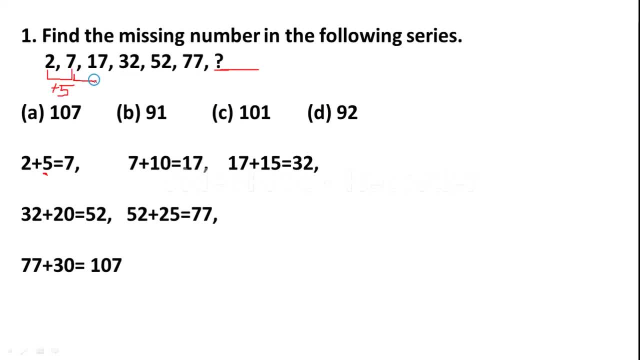 That is 2.. Ok, 2 plus 5, 7.. Next, 7 plus 17 is Ok. they have added again 10.. 10 plus 10, then 17 to Ok. 7 plus 10 is 17.. 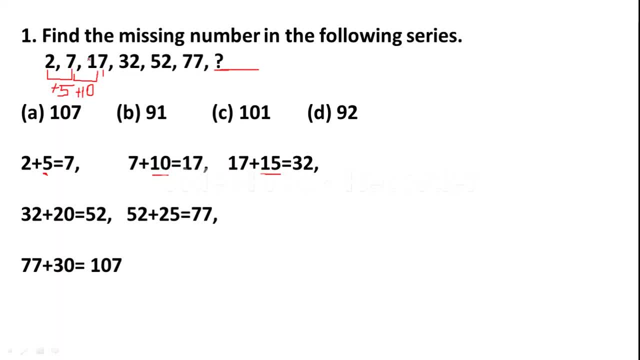 Then 17 plus 15 is 32.. Here they have added 15.. Ok, next, 32 plus 20 is 52. Again, they have added 20.. And 52 plus 25 is 77. So again here they have added 27.. 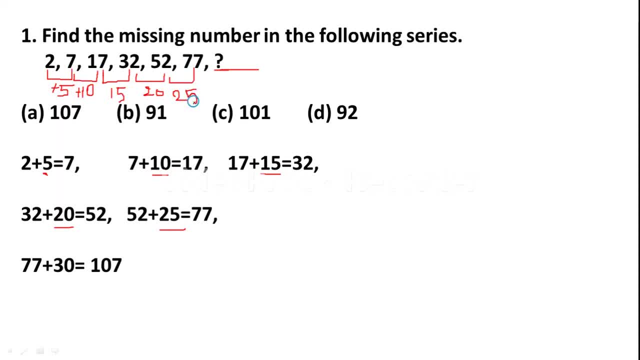 25.. Ok, see here, friends, here they have added 5. in the next they have added 10. next they have added 15,, 20,, 25.. So in the next series we should add 30. Because here the difference is 5. So 25 plus 5 is 30. So we should add 30. So 77 plus 30 is 107.. So the correct answer for this question is: 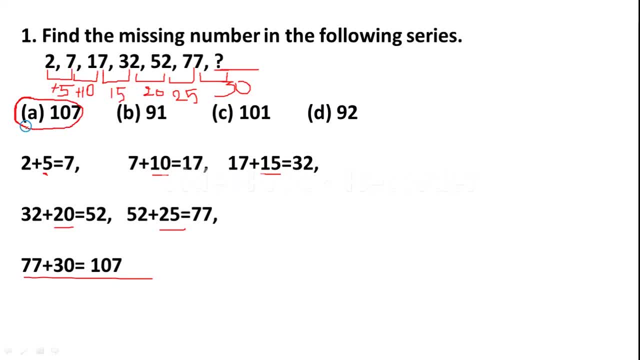 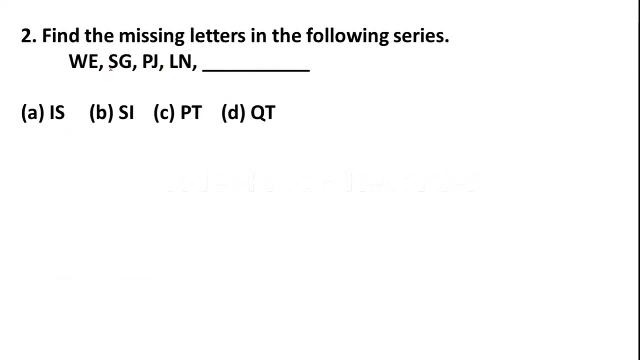 option A 107 is the right answer. Friends, I hope you got this. Please practice more and more questions on this. If you have any questions, you can ask me in the comment box. Friends, let us go to the next question. Find the missing letters in the following series: W, E, S, G, P, G, L, N- and we have to find the next series. Ok, friends, options are: option A, IS, option B, SI. 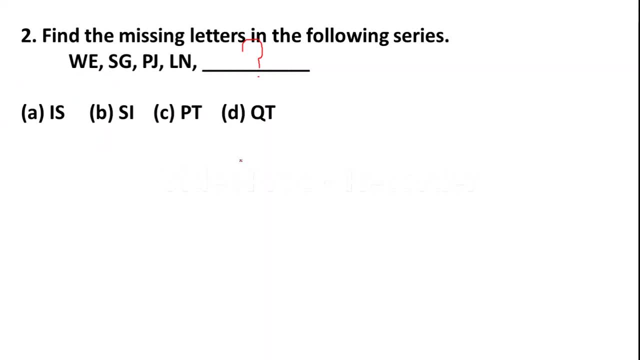 Option C, P, T. Option D, Q, T. Friends, first we will write the alphabets and we will assign the numbers. It will be easy to find out. Ok, Friends, in every series let us write the first alphabet, Ok. 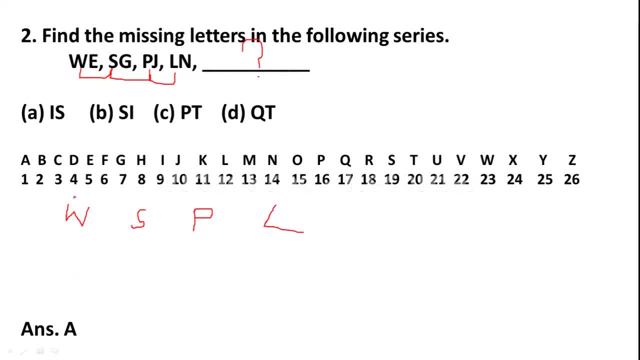 And L Friends. see here where is W. W is at 23rd position and S is at 19th position. Ok, They are coming backward. W to S, The difference is 1,, 2,, 3 and 4.. So here the difference is minus 4.. And again, S to P. 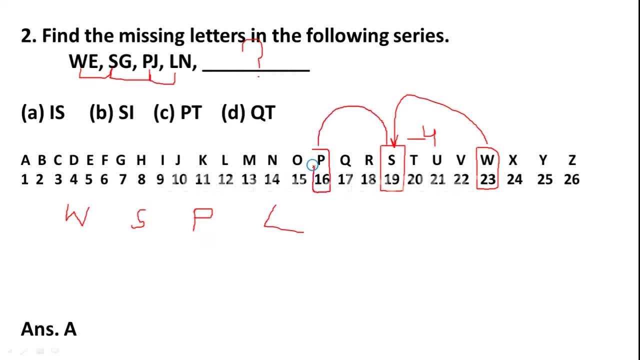 S is at 16th position. It means the difference is minus 3.. Then P to L, Friends, again from P to L, the difference is 1, 2, 3, 4, again minus 4.. I think you have got the pattern here: Minus 4,, minus 3,, minus 4.. Then next is minus 3.. 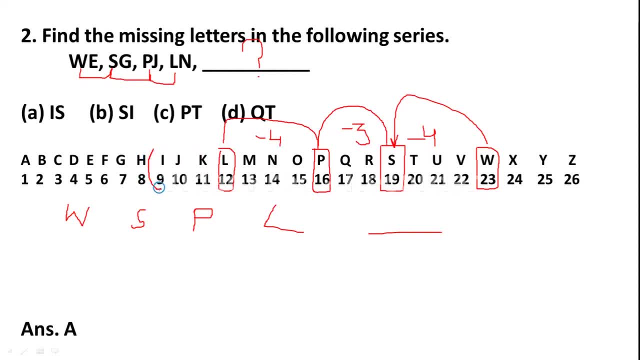 3. 1.. 2, 3. so the next alphabet will be I. so minus 3. so the next alphabet is I. okay, now let us take second alphabets from each series: E, G, J and N. okay, let us see E, G, J and N. we should find the next alphabet. okay, very G friends, here is the. 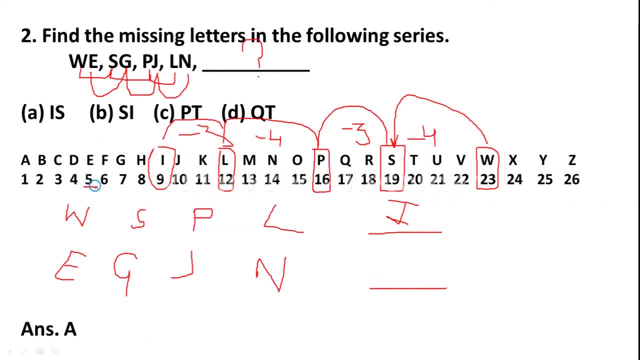 okay, next, next G. here what they have did, they have done here they have added plus 2. it means here g, the difference is plus 2. now, next from G to J: G to J: again 1, 2, 3, again the difference is plus 3,. J to N: 1, 2, 3,. 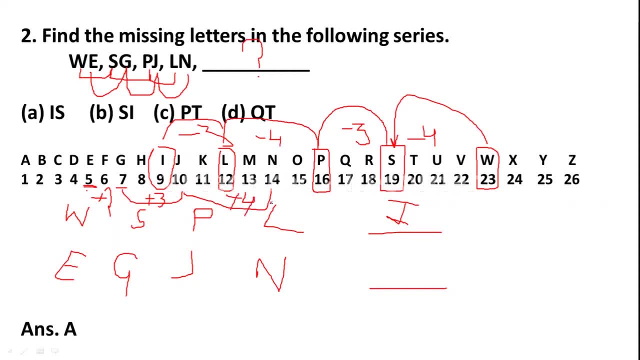 4,. the difference is 4,. ok, the next difference will be 5,. so 1,, 2,, 3,, 4,, 5, it is yes, so the next series is yes, so I S is the correct answer. so here the option A is the right. 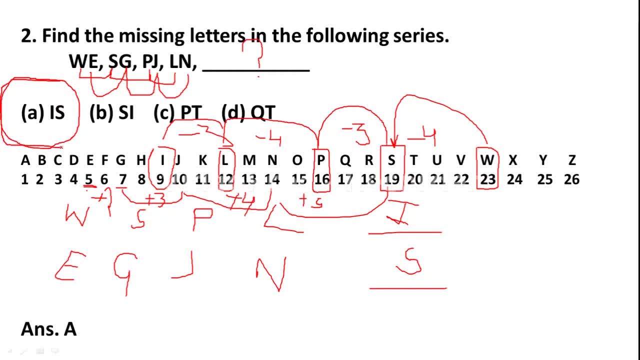 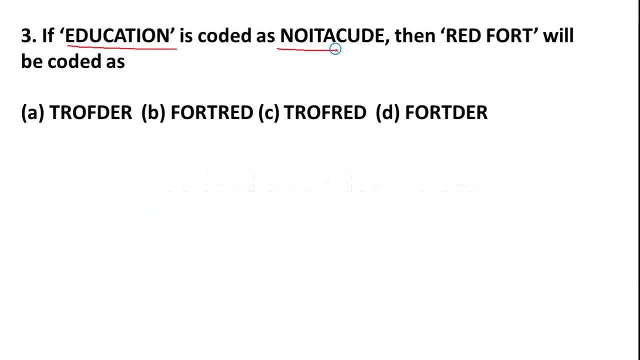 answer. I hope you understood this. now we will go to the next question, friends here. the third question is: education is coded as N, O, I, T, E, C, U, D, E, then red port will be coded as options are given here. four options are there. ok, let us see, friends. 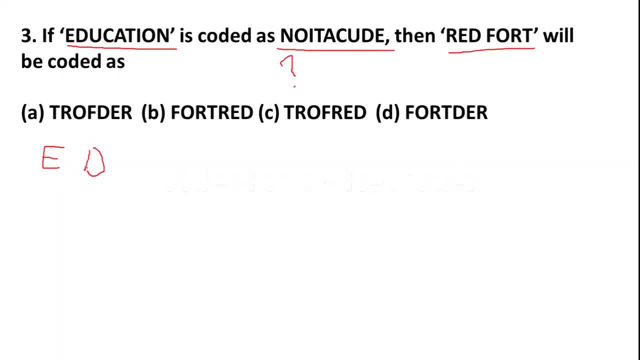 let us understand the pattern Pattern plus first pattern, we will see education is written as N O, I, T, E, C U, D, friends here. just the code is the reverse of the given word. the word is education. just they have. 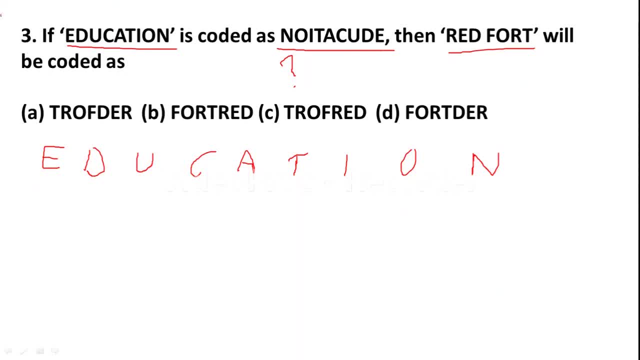 written it in the reverse order. In place of E they have written N, means E is at the first word, the last word is N. the last word is written at the first place, next O. at the second place, I, next T, next. 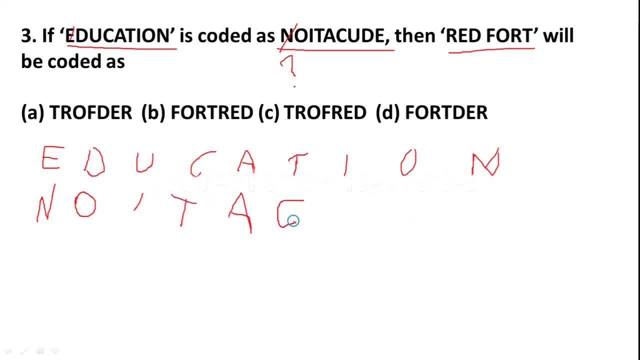 A, then this C here, then U D And E N O I T E C U D. ok. now, in the same way, we have to write red port R E D F O R T, ok. 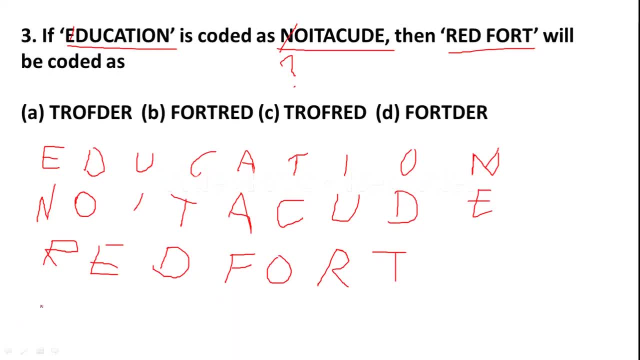 At the end point And T is there, so we will write it at first T, then R, then O F D E R. So the answer is T R O F D E R. 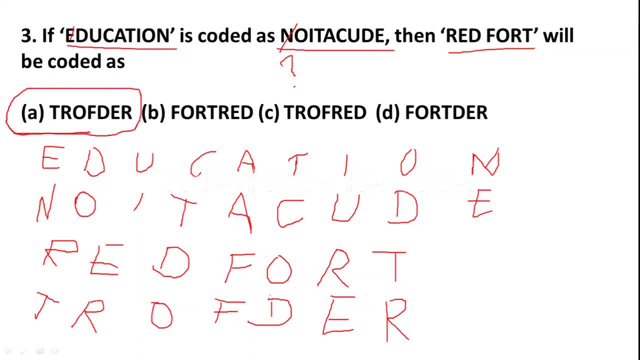 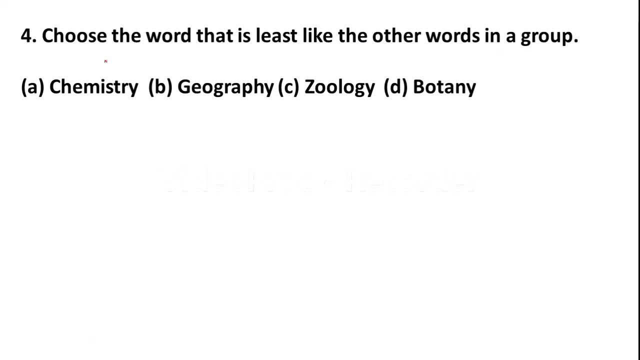 So option A, T, R, O, F, D, E, R is the correct answer. I think you understood this. Let us see the next question. Choose the word that is least like the other words in a group. The words are: option E- chemistry. option B- geography. option C- geology. option D. 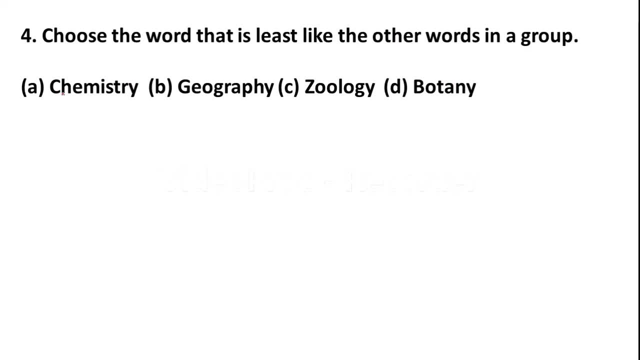 botany. I think easily. you can guess it: chemistry, geology, botany are the branches of science, but geography is not the branch of science. So here the correct answer is option B is the right answer: geography. Ok, Let us go to the next question. 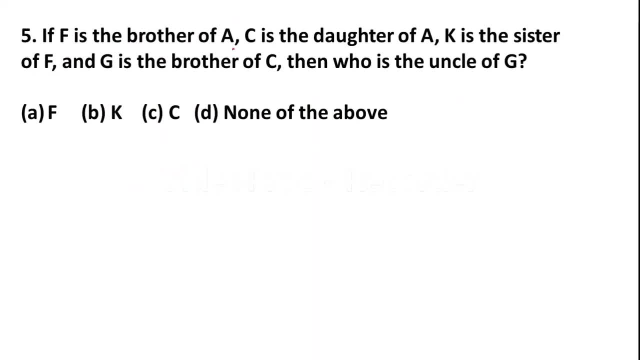 Friends, if F is the brother of A, C is the daughter of A, K is the sister of F and G is the brother of C, then who is the uncle of G? Options are: F, K, C, none of the above. 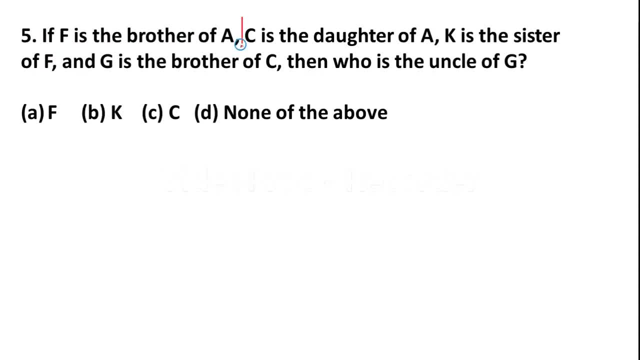 Ok, Friends, if the F is the brother of A, Ok, We will write F here. F is the brother means he is male, F is the brother of A. Next, C is the daughter of A. C is the daughter of A. Ok, 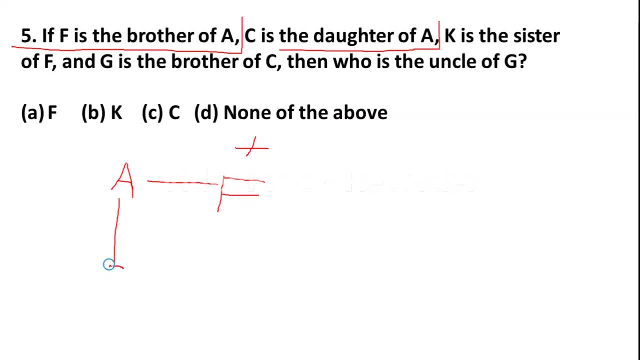 C is the daughter of A. Ok, Ok, C is the brother of A. For female, we will give minus sign. Next, K is the sister of F, K is the sister of F. Ok. K is the sister of F And G is the brother of C. Ok. 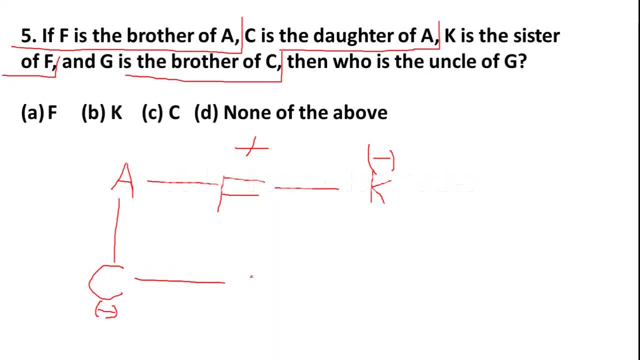 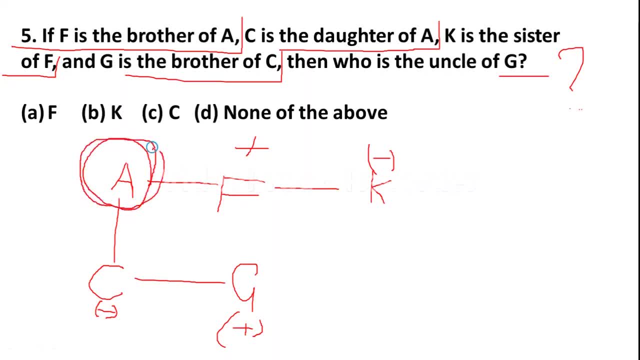 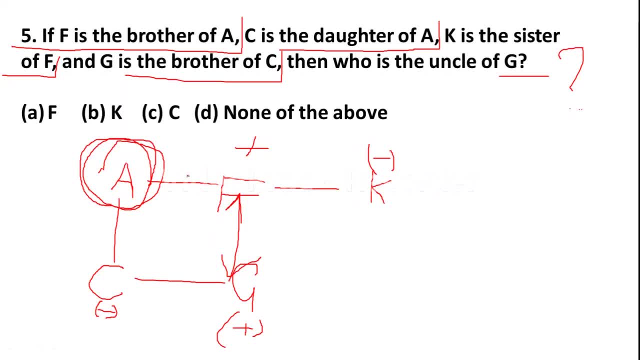 Then who is the uncle of G here? K is not, because K is female. So F is the uncle of G. So here option A is the option A. F is the correct answer. I think you understood this. Now let us go to the next question. 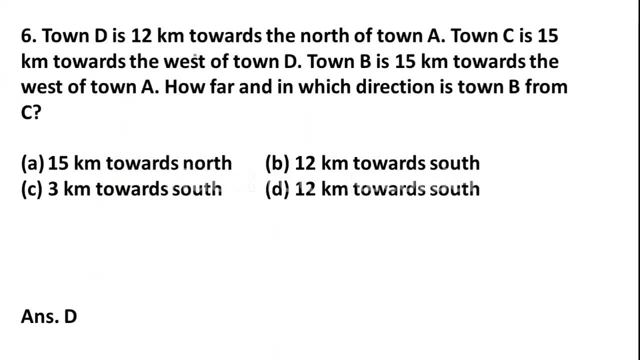 So, friends, town D is 12 km towards the north of town A. Town C is 15 km towards the west of town D. Town B is 15 km towards the west of town A. How far and in which direction is town B from C? 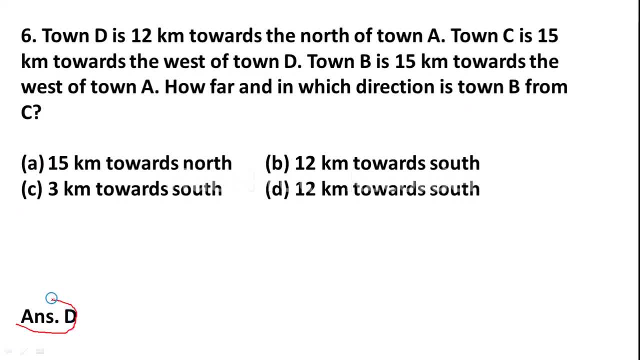 Ok, let us see the answer. friends, by mistake The answer is given here, option D. But let us solve it. Ok, first we will mark No North east, south west. Ok, town D is 12 km. town D is 12 km towards north of town A. Ok, here we will write town A, Then towards north of town A. 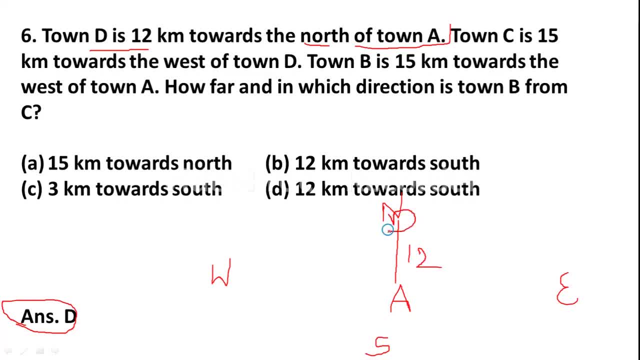 12 km. D is there. Next town C is 15 km towards west of D. Ok town C is 15 km towards west Town C. ok Town C 15 km towards west. Next town B Town B is 15 km towards west of town A Of town A towards west. it is 15 km. 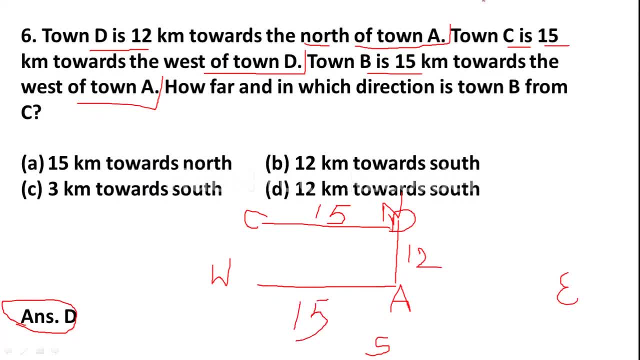 Ok, now the question is: how far and in which direction is town B from town C? Ok, here, town B is there. Here, town C, Town C is there. See, here it is a square. These both sides are 15 km. 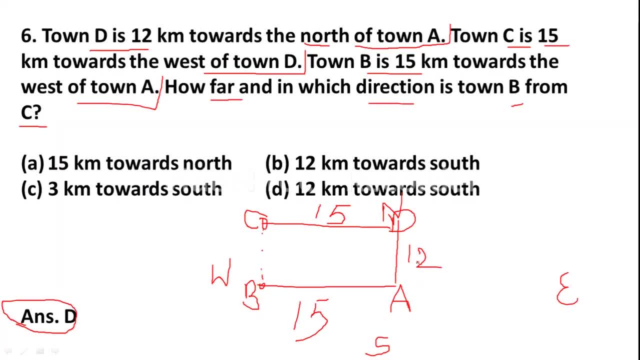 15,. ok, Then this side also. D A distance is 12.. So C B distance is also 12.. Here in two options: 12 is there, So easily we can eliminate two options here. Ok, next question is: in which direction? 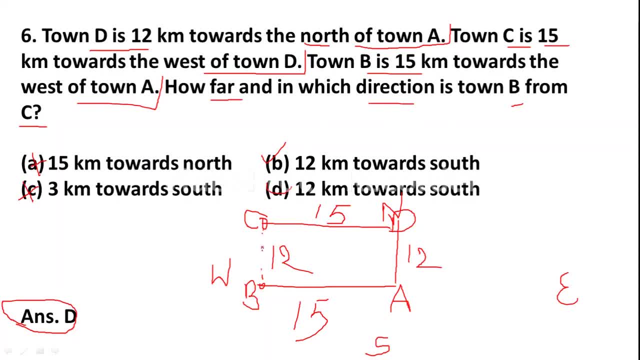 Ok, from which town B? from town C Means from town C. It is at the direction of south, So here answer D is the correct answer. Ok, friends, by mistake both the options are same here. Ok, don't worry. 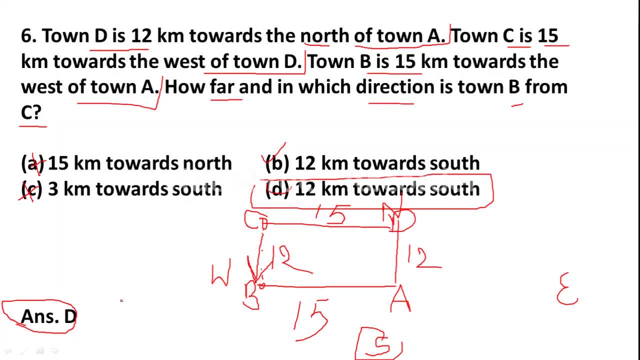 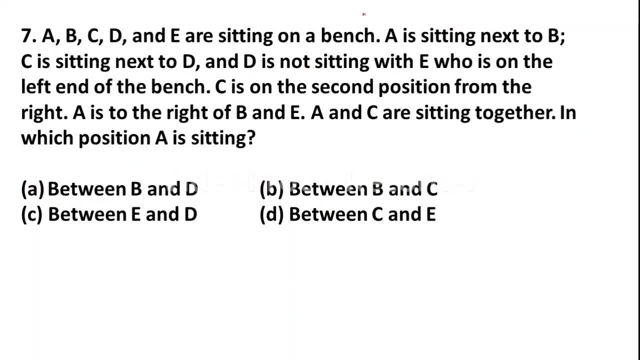 I hope you got it. how to solve it. Let us go to the next question. Friends A, B, C, D, E are sitting on a bench. We will solve it while reading the question. Ok, A, B, C, D. 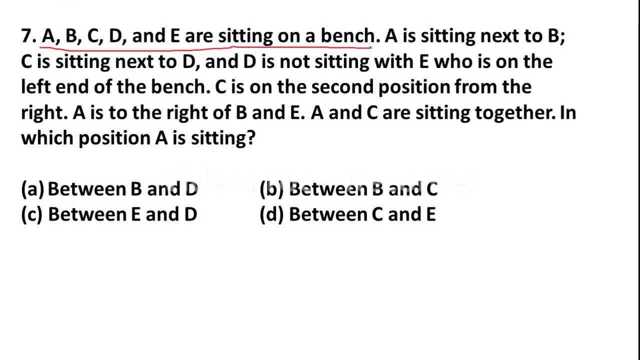 And E are sitting on a bench. A is sitting next to B- Ok, A is sitting next to B, Ok, here. B is there. Then here A is there. Next. C is sitting next to D- Ok, we will write it later. 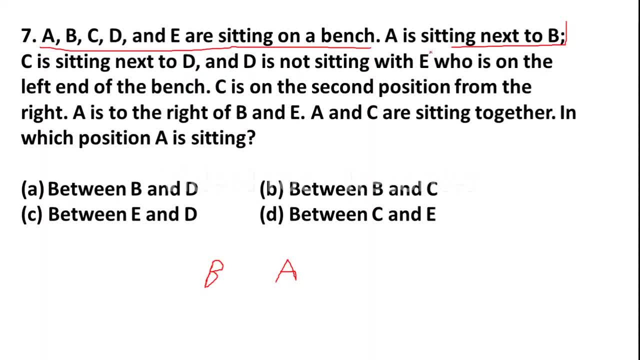 That D is not sitting with E. Ok, D is not sitting with E. Who is on the left end of the bench? Ok, E is at the left end of the bench And he is not sitting with D. Next question is: C is on the second position. 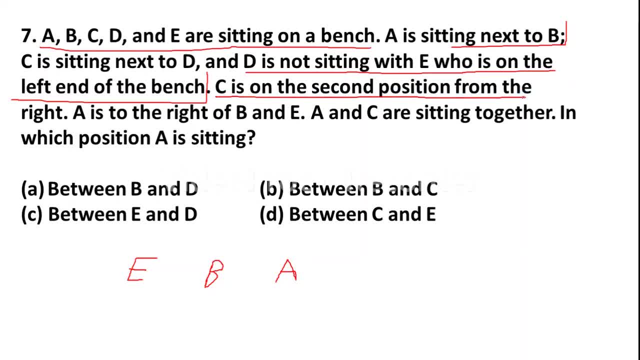 C is on the second position from right. Ok, C is on the second position. Means C: Ok here. C is there. He is at the second position. Means here, someone is sitting here. Ok, now, who is sitting here? 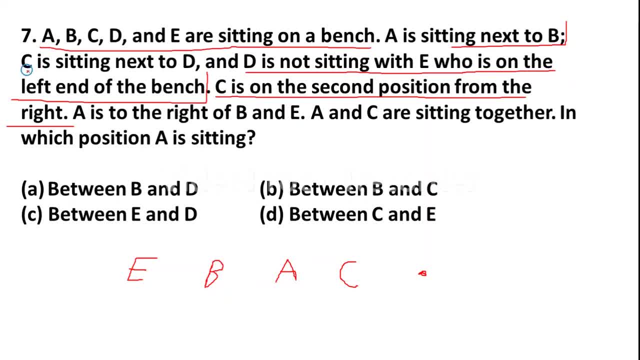 Ok, next C is sitting next to D. Ok, here D is sitting, Then here D will come Next. A is to the right of B and E. Ok, A is to the right of B and E, It is right. 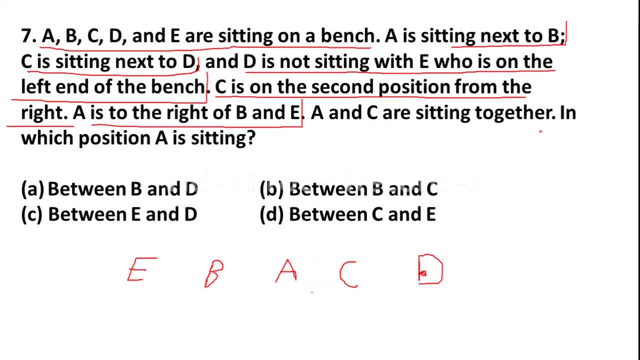 Then A and C are sitting together. A and C are sitting together. Yes, this is also right. Ok, in which position A is sitting now? Option A: between B and D, B and D. wrong Option B, B and C. 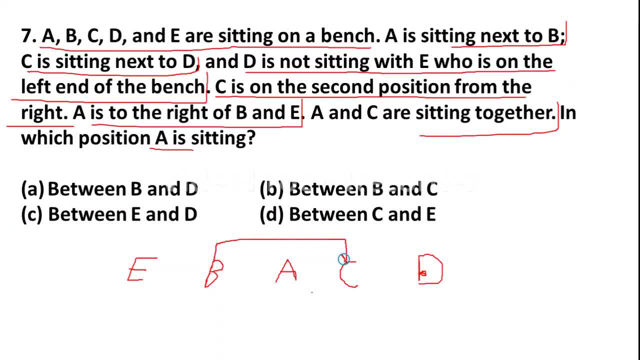 Yes, A is sitting between B and C, So option B is the correct answer. Friends, you have to solve more and more questions to B family, So let us go to the next question. So let us go to the next question. 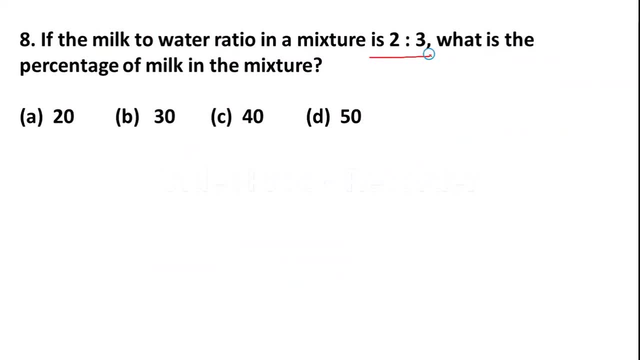 If the milk to water ratio in a mixture is 2 to 3, what is the percentage of milk in the mixture? Very easy question, Friends, to solve this. there are total. how many parts are there? 2 parts is milk and 3 parts is water. 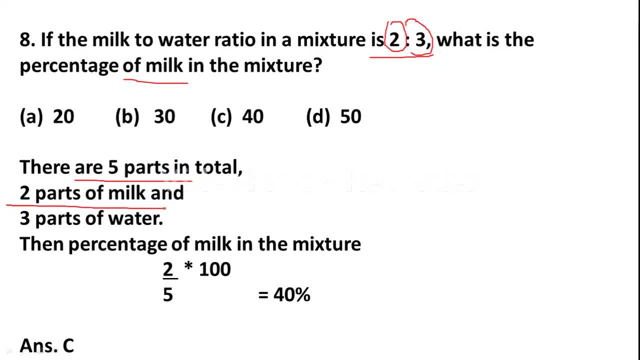 So total 5 parts are there 2 parts of milk, 3 parts of water, Then the percentage of milk. So the percentage of milk is equal to the percentage of milk is 2.. Total parts is 2 plus 3, 5.. 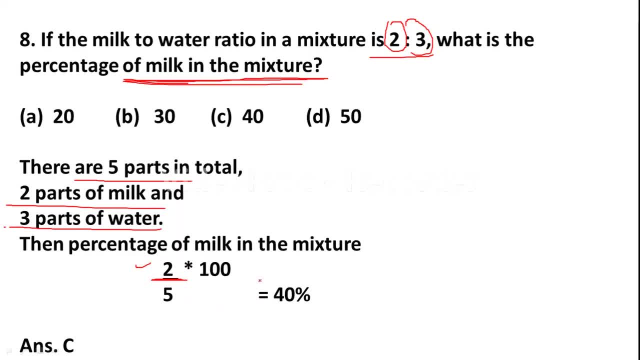 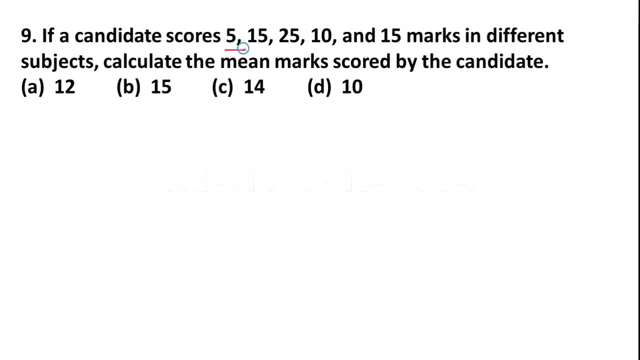 So 2 divided by 5 multiplied by 100 is 40%. So here the correct answer is option C. 40% is the correct answer. Very basic level question. So let us go to the next question. If candidate scores 5,, 10,, 15, 25,, 10,, 9, 15 marks in a different subject. 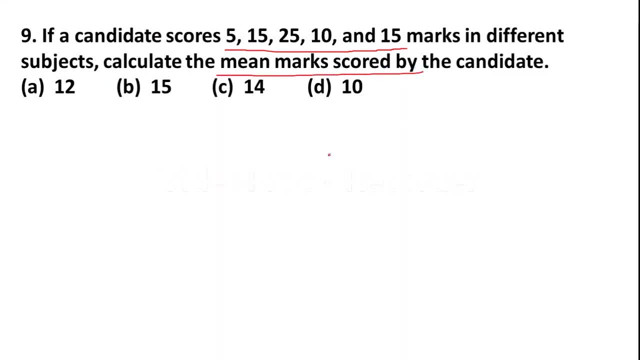 calculate mean marks score obtained by the candidate. Mean is equal to mean is denoted as x. bar Mean is equal to sigma x divided by n, where sigma x is sum of all given observations. n is number of observations. n is number of observations. 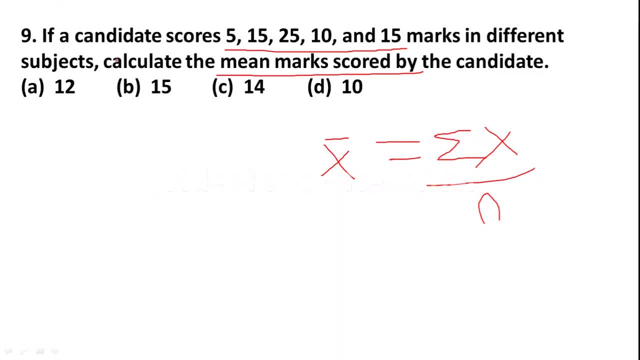 Okay, no need to remember the formula. also, friends, Easily you can calculate. Okay, how to calculate it: 5 plus 15 plus 25 plus 10 plus 15 divided by 5.. So it is 70 divided by 5,. 14 is the right answer. 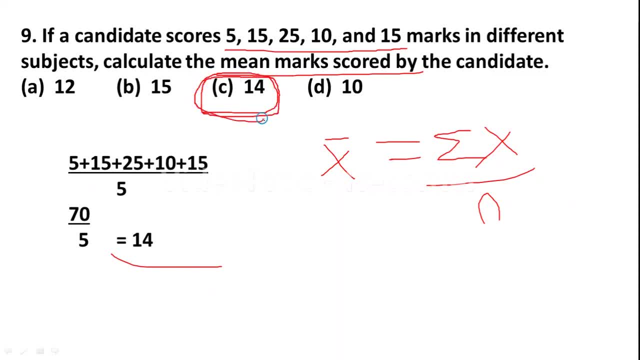 So option C is the correct answer. 5 means here 5 observations are there: 1,, 2,, 3,, 4 and 5.. 70, the sum of all given observations. I hope you understood This. and here the correct answer is option C 14.. 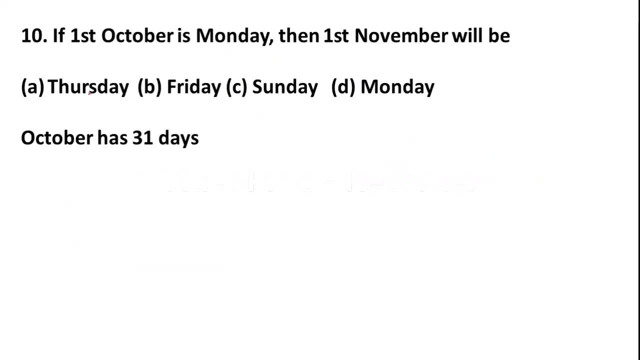 Now we will see the next question. Friends, if 1st October is Monday, then 1st November will be Thursday, Friday, Sunday, Monday. Okay, friends, remember October has 31 days. Yeah, we know, October has 31 days. 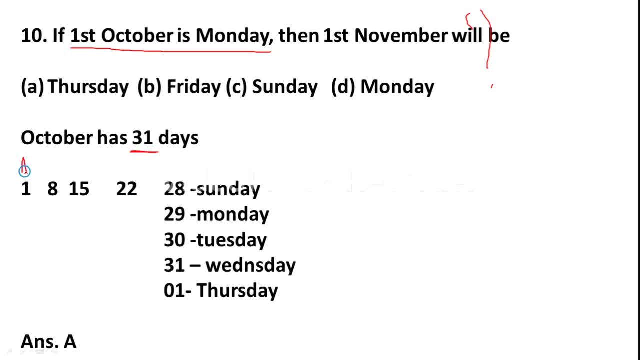 And 1st October. 1st October is Monday. Okay, they have given here: 1st October is Monday. After 7 days, again Monday will come. It means 1st is Monday, 2nd is Tuesday, 3rd is Wednesday, 4th is Thursday, 5th is Friday, 6th is Saturday, 7th is Sunday. 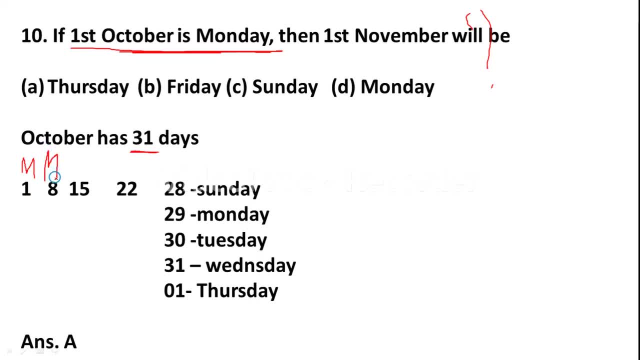 Again. 8th is Monday. Okay, again 15.. 5th is Monday Again. 22 is Monday 23,, Tuesday 24,, Wednesday 25,, Thursday 26,, Friday 27,, Saturday 28,, Sunday 29,, Monday. 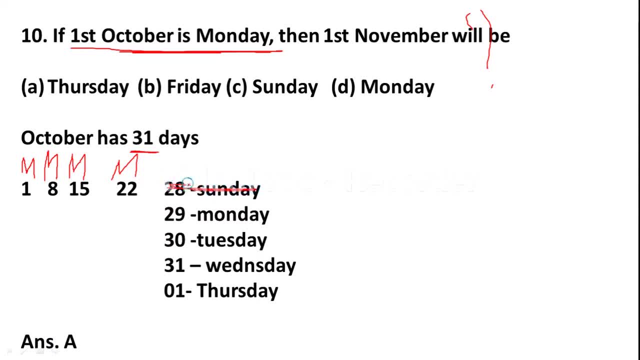 Again this: it is okay if you won't write also 29,. again, 29 is, So 30 is Tuesday, 31 is Wednesday, so next November 1 will be Thursday, So option A is correct. is the correct answer. 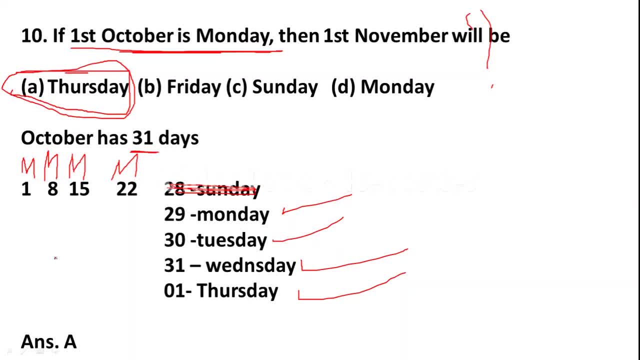 I hope you understood this, Friends. let me explain you once again Here. October has 31 days and 1st October is Monday. So 8th October is also Monday, 15th October is also Monday. 15th October is also Monday. 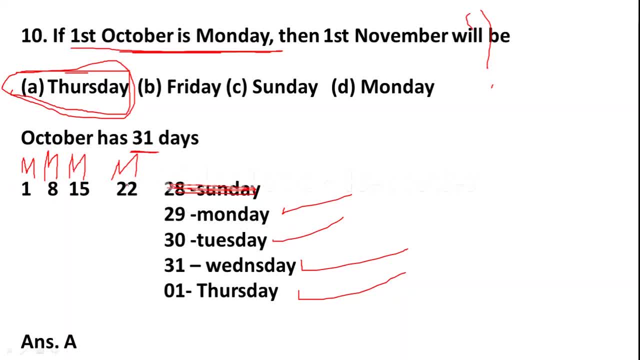 So 22 October is also Monday and 29th October is also Monday, so 30 is Tuesday, 31 is Wednesday and after Wednesday, after 31,. November 1 will come, so after Wednesday Thursday will come, so the next day will be Thursday. 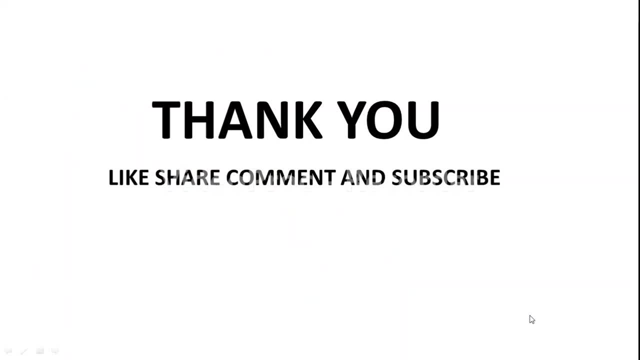 Option A is the correct answer. Friends, thank you very much. Thank you for watching this video And to get the 20 mocktail series, go to our website and enroll for the mocktail series. Thank you, Join the crew. 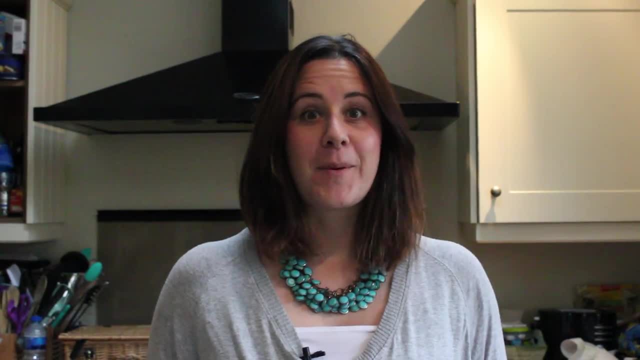 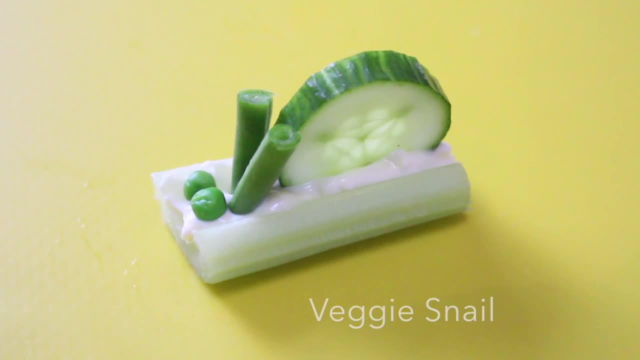 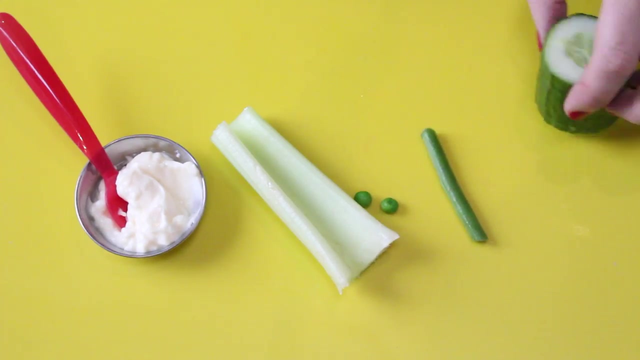 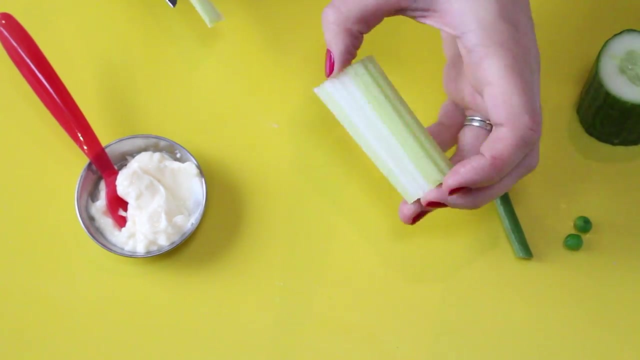 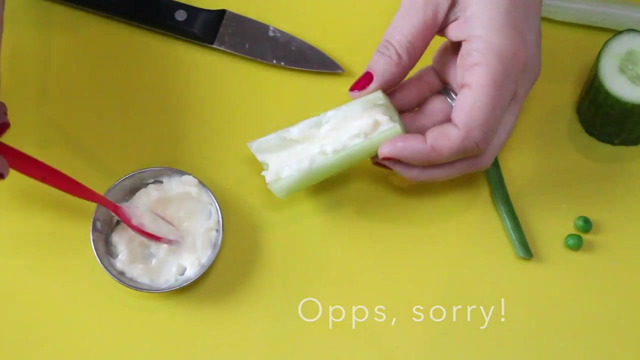 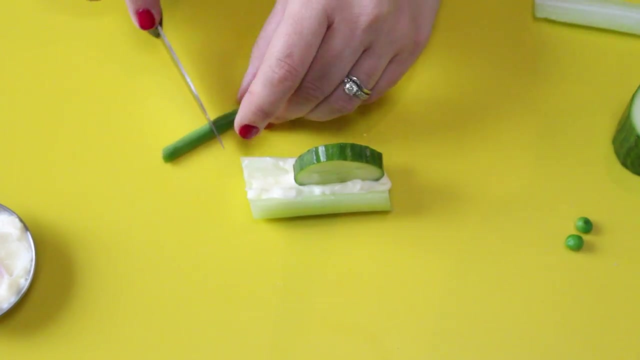 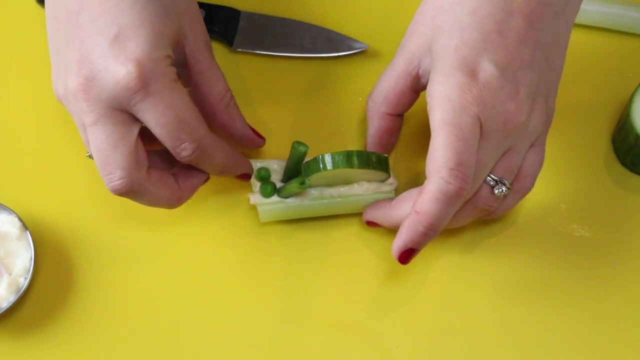 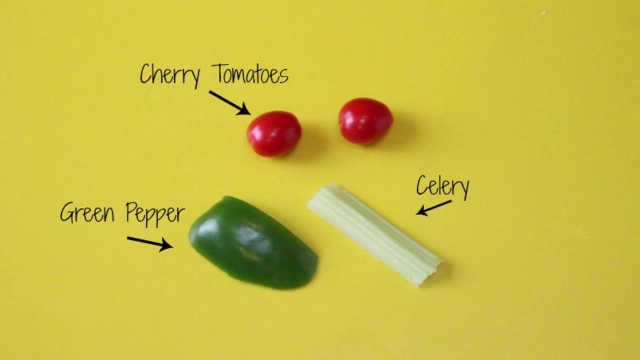 Hi, I'm Ciara from MyFossilEatercom. If you have trouble getting your kids to eat veggies, then stay tuned, because I have a really fun and simple snack for you to try today. Hi, I'm Ciara from MyFossilEatercom. If you have trouble getting your kids to eat veggies, 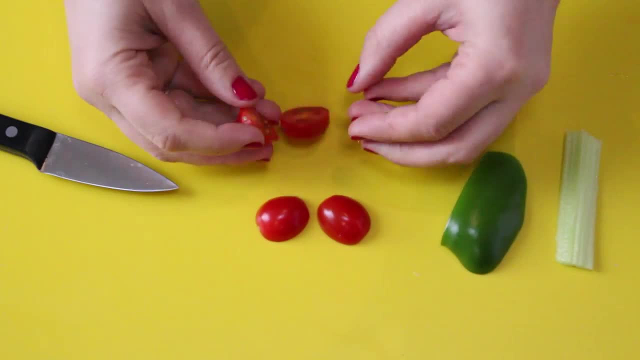 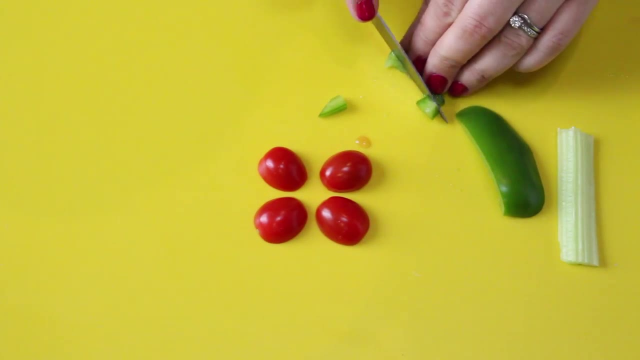 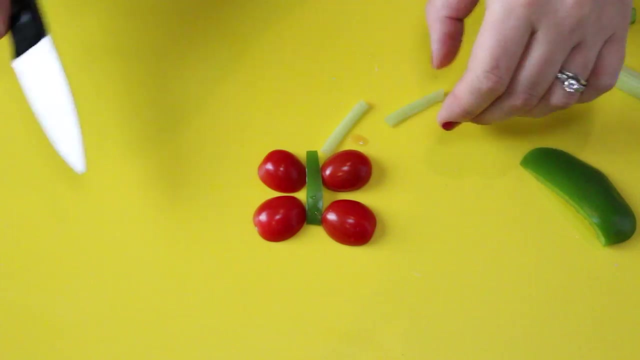 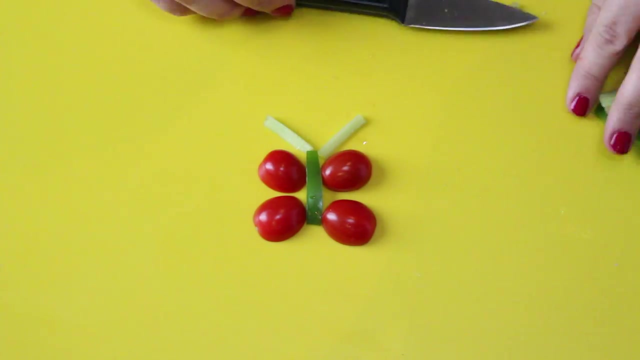 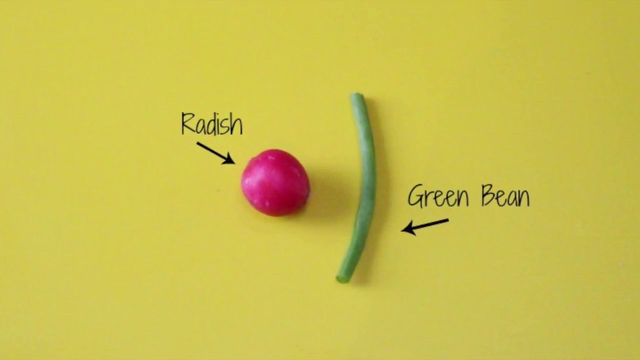 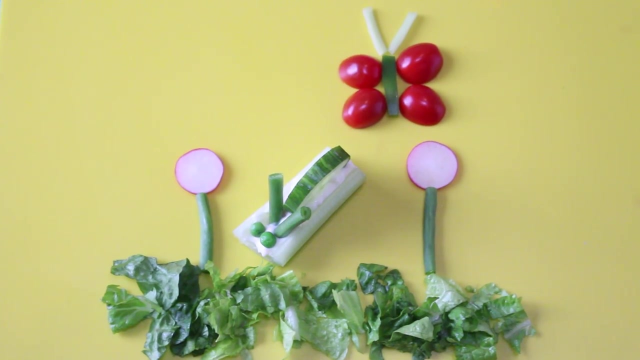 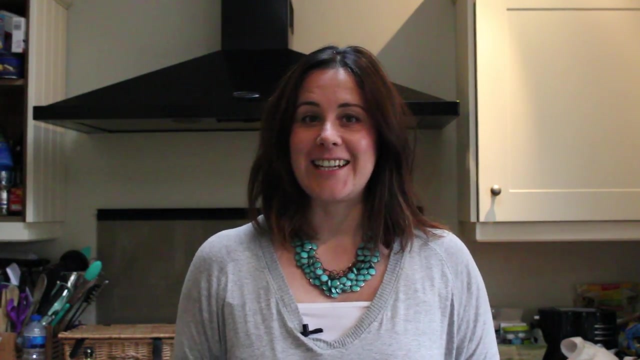 then stay tuned, because I have a really fun and simple snack for you to try today. I hope you enjoyed this really fun snack for kids. If you did, please do give it a thumbs up. Also, let me know in the comment section below what kind of ways you get your.